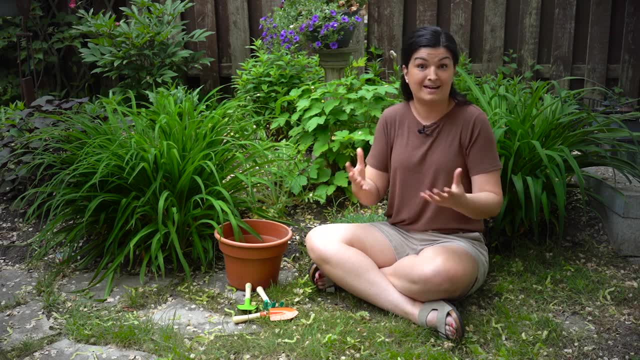 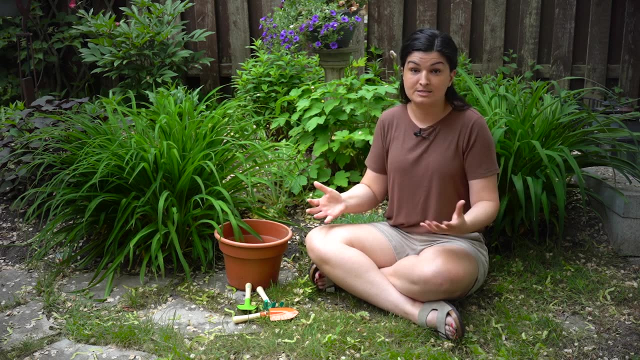 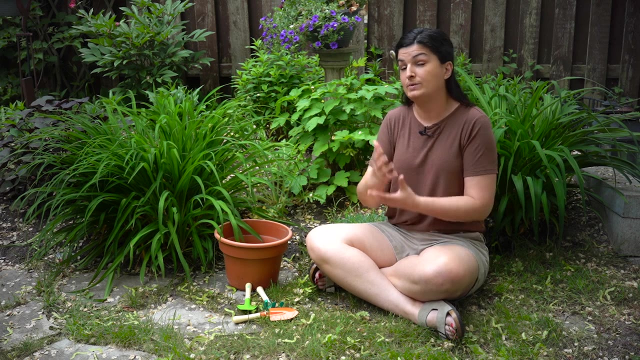 that sense of ownership to be responsible for something that is theirs. so take a trip to your local nursery or garden center and pick out some nice plants for them that they can then be responsible for. so with that, you're giving them the responsibility of watering it, so you can give 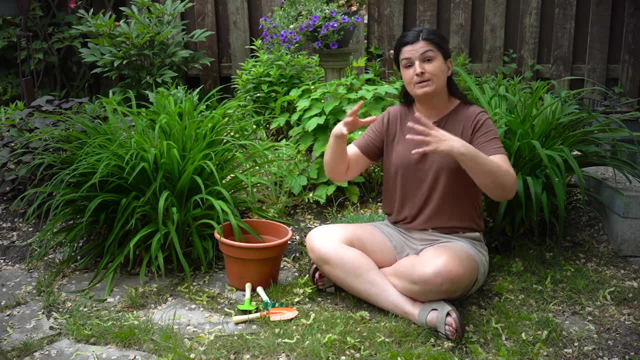 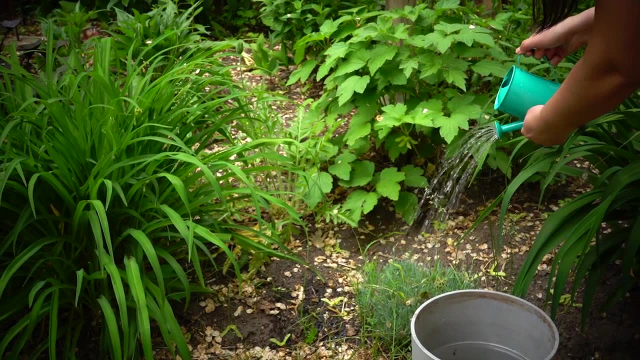 them access to the hose, if you have one, or simply have a bucket full of water that they can dunk their watering can into. you want to use a child-sized watering can, one that they're going to be able to maneuver, so that they can then water their plants- another really fun activity that you 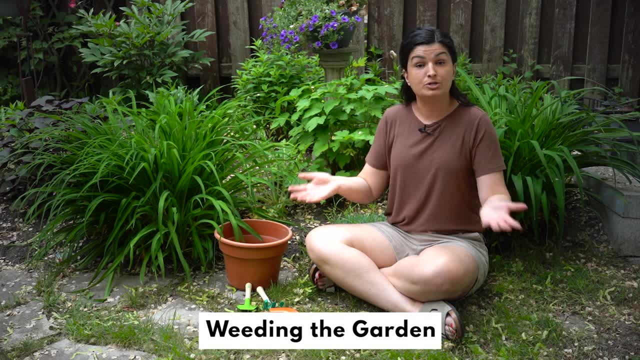 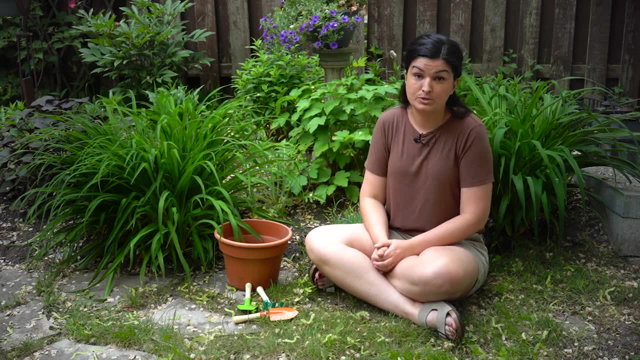 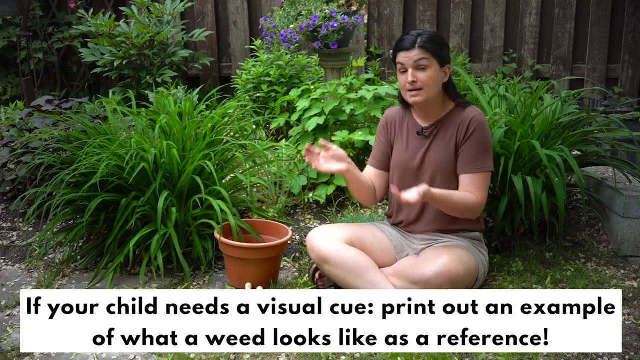 can do with a preschool age child is weeding the garden. you can show them the difference between the flowers and the weeds, give them a child-sized tool and invite them to help you to weed the garden. something that you could also do if your child needs more of a visual cue is you can even take pictures of the weeds and laminate them. 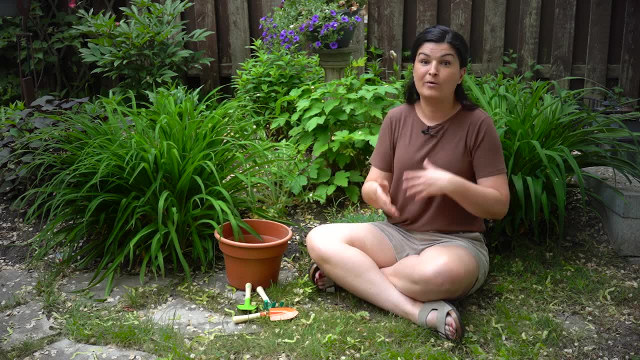 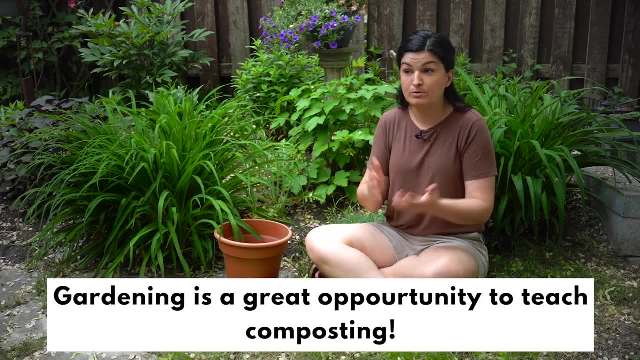 and then your child has that as a reference point so that they know what exactly they are are weeding versus what needs to stay in the garden. at this age, you can also teach your child to compost. you can take your scraps of food, of the fruits and vegetables from your meals and have an area of 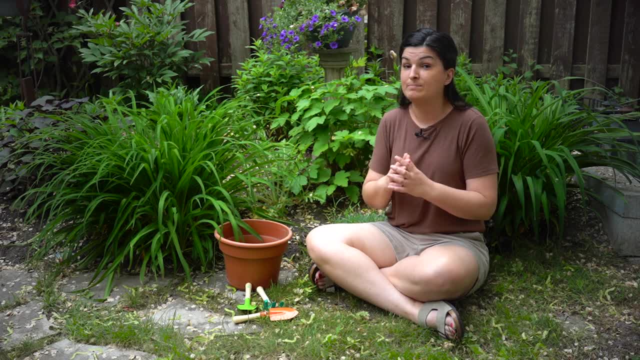 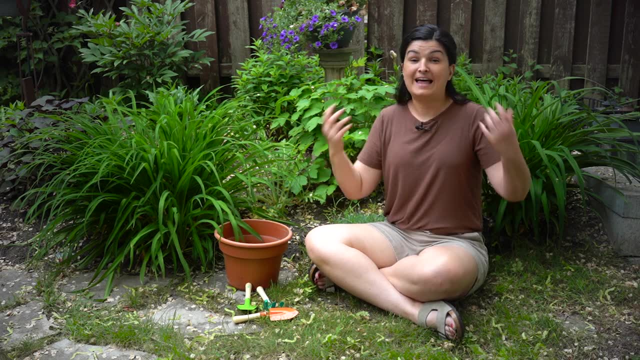 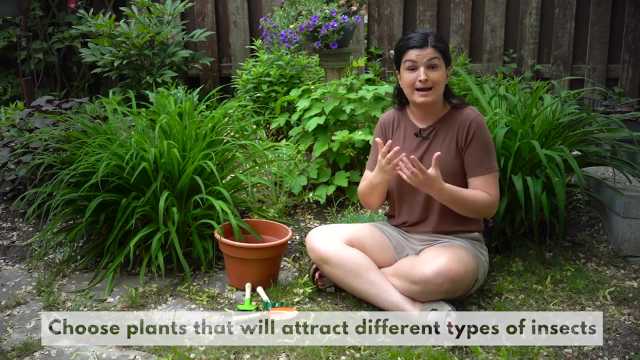 your garden where they can compost. it's a really neat activity for them because the worms come and have a wonderful learning opportunity for them. and then, lastly, I would recommend, if you are planting a garden like this, a really big lush garden- is to choose plants that are going to attract different 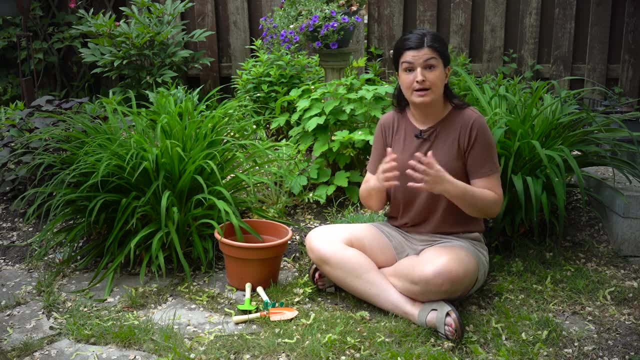 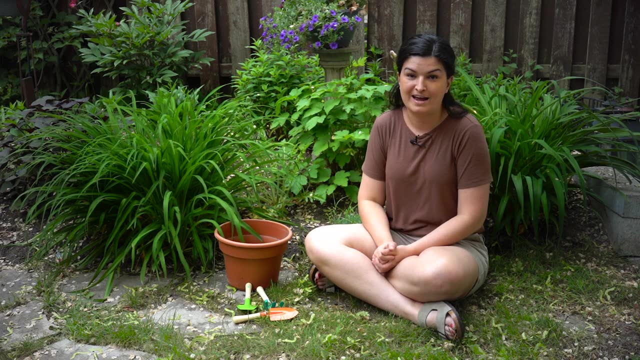 types of insects, so plant flowers that are going to attract butterflies, bumblebees, all those types of things, so that your child can really see everything that a garden has to offer and it's really going to enrich their learning just to be able to observe it and be a part of it. if you're 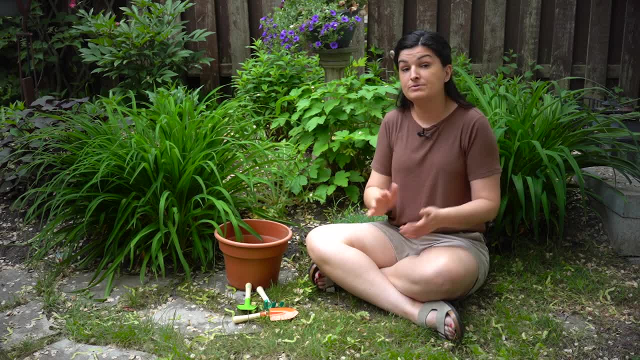 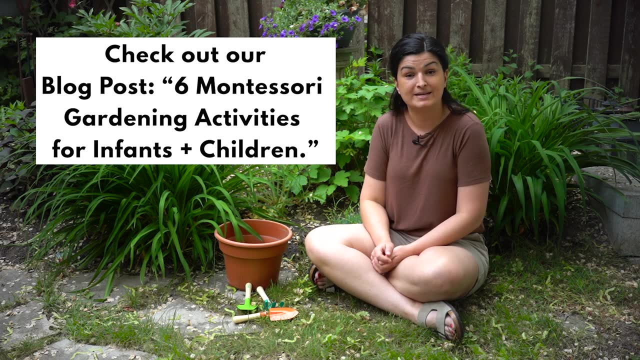 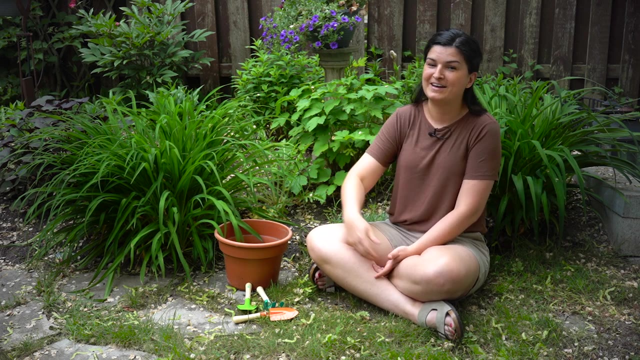 interested in learning about some of the developmental benefits gardening for young children. we have a blog post titled six Montessori gardening activities for infants and children and I will link to it in the description below. I hope you found today's video helpful. I hope you enjoy gardening with your children and I'll see you next time. bye, thanks. 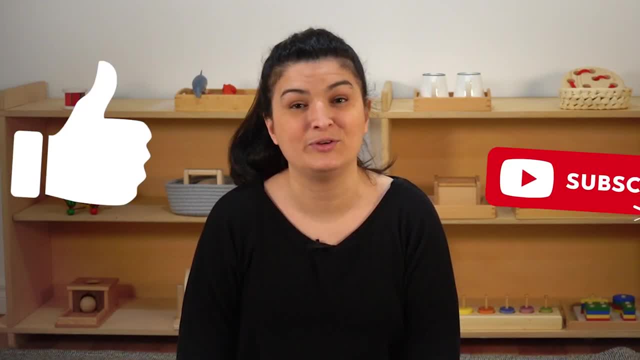 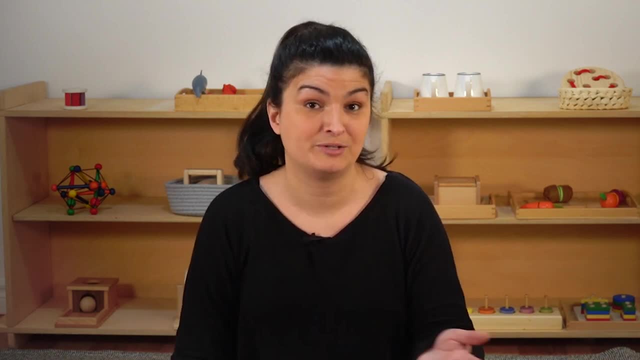 for watching. if you liked this video, it really helps our channel. if you like and subscribe, this helps other parents to find our channel and if you have a question, feel free to comment your question below and we'll answer it in a future video. take care, bye. 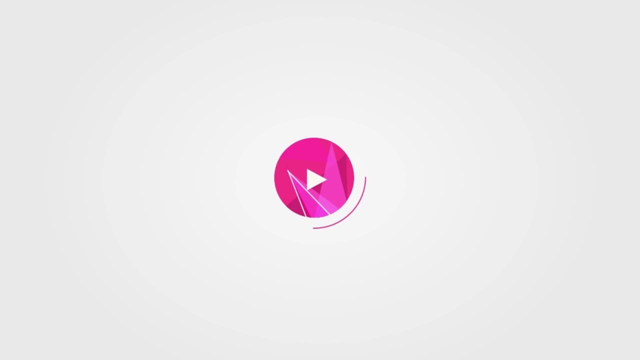 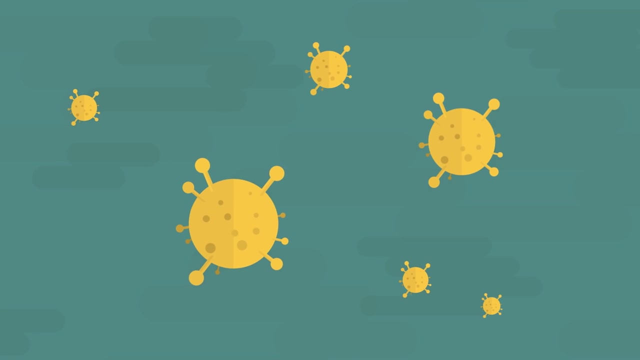 A lot of waste is produced on a global scale. Unless the waste is recycled, it fills up in our landfills, destroys habitats and will be a very serious health hazard. Imagine if one day the waste that we produce can be naturally broken down by microbes in the environment. 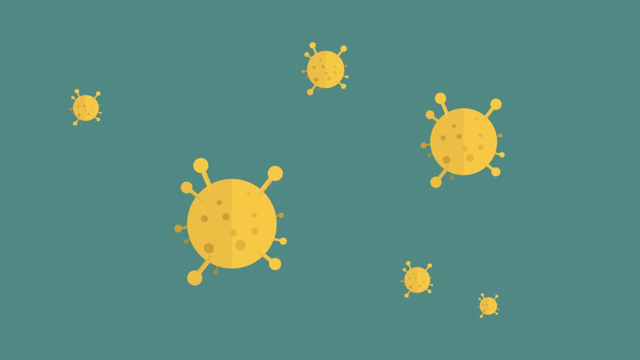 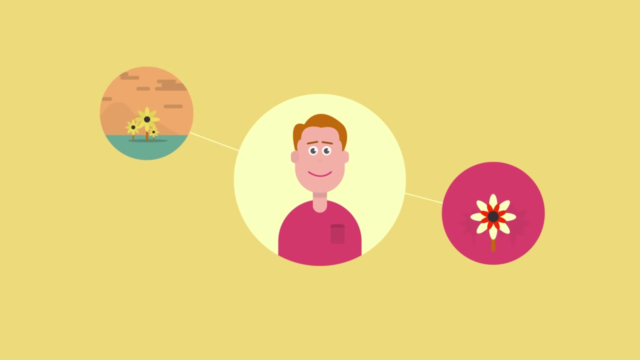 or dissolve into safer materials. This principle explores such a concept. Ideally, whatever we use and throw away would present no hazard to the environment and would not accumulate in landfills. If you've ever had to get stitches because of an injury, the stitches slowly. 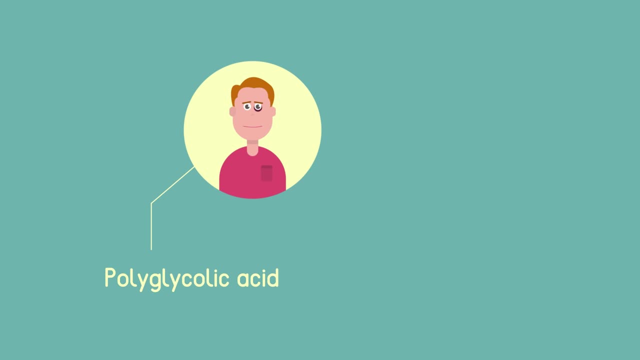 dissolve over time. This is, in fact, a polymer called polyglycolic acid, which is broken down into its respective monomers by enzymes in our body. This is then either respired as carbon dioxide or excreted in our urine. There is a new class of plastics known as 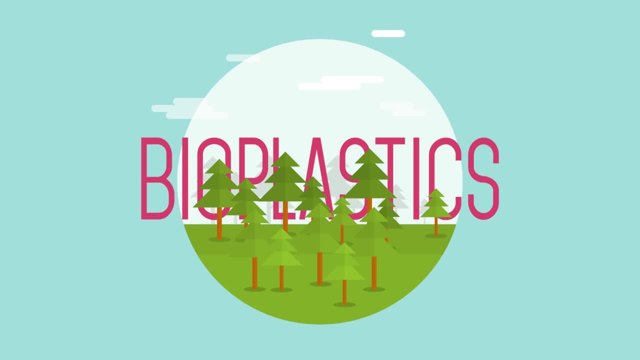 the bioplastics. These polymers are made from natural monomers such as cellulose and lactic acid and can be broken down in the environment. For more information on these, please see our Synthetic Polymers video. As a result of these bioplastics, carrier bags can be. 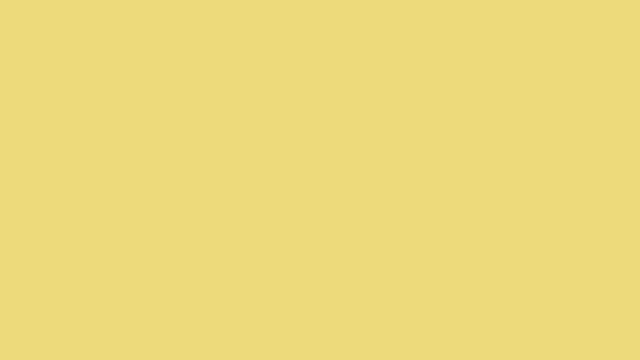 broken apart by microbes in the environment. This is important because it reduces the amount of waste that accumulates in landfills. Ache cartons, once made of polystyrene, which is derived from petroleum-based products, are now usually packaged in recycled newspaper material which can be recycled and therefore do not.